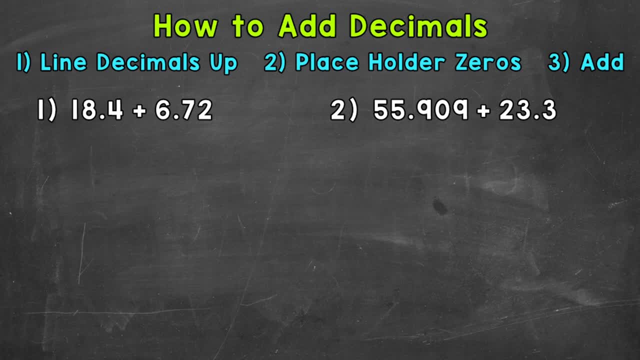 That's going to line up all of our places. So, number one, we're going to do 18 and 4 tenths plus 6 and 72 hundredths. Notice how the decimals are lined up Now. it may look a little offset there, but we can use placeholder zeros to better align this. 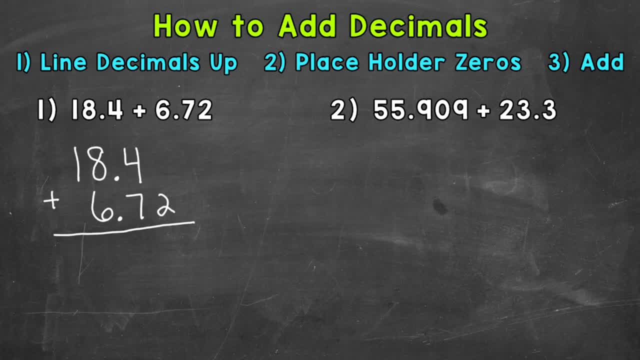 and make it look a little more organized. Meaning 18 and 4 tenths. we can put a zero in the hundredths place. That way we look a little more lined up. Remember: zeros to the right of a decimal do not change the value. 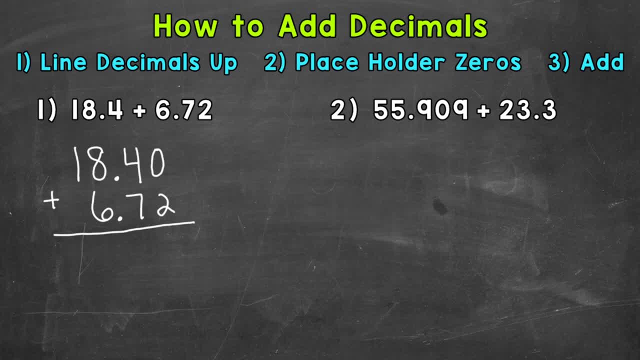 That's an equivalent decimal, so we are able to do that. We're not changing the value of the problem. Once we're done with that, we're going to go ahead and set up our problems. Once we have that, we add. 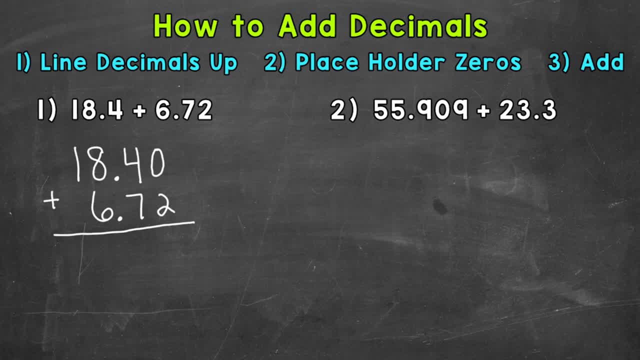 Start with the hundredths place, So 0 plus 2 is 2.. Then we move to the tenths place: 4 plus 7 is 11.. So put our 1 and regroup, or carry there. Now bring our decimal straight down. 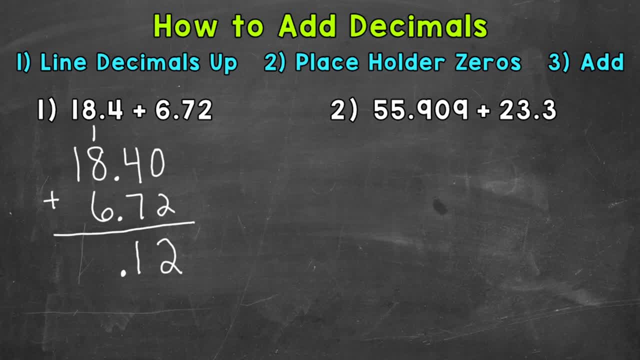 It's lined up throughout the entire problem. Now we add the ones: 1 plus 8 is 9.. Plus 6 is 15.. Regroup or carry the 1.. Now we add the tenths place: 1 plus 1 is 2.. 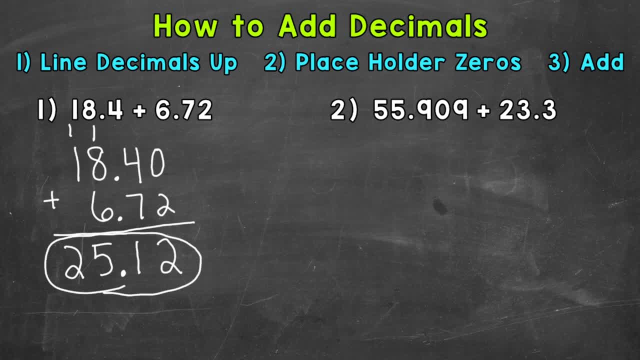 So we get 25 and 12 hundredths. To recap, as far as where we put the decimal in our answer, the decimal should be lined up throughout the entire problem, So we bring it straight down Now. before I move on to number 2,, I do want to mention a common mistake. 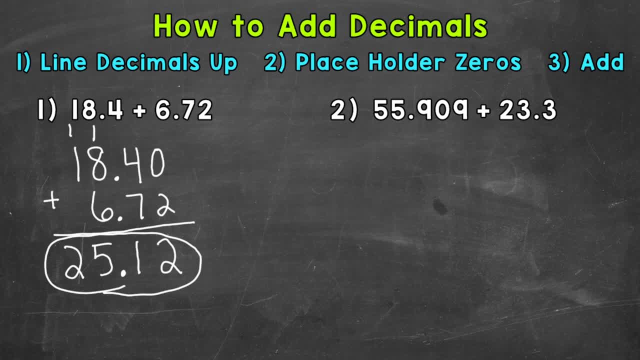 And that's going to be lining the digits up, Meaning for number 1, it would look like this: 18 and 4 tenths plus 6 and 72 hundredths, So 3 digits lined up with 3 digits. 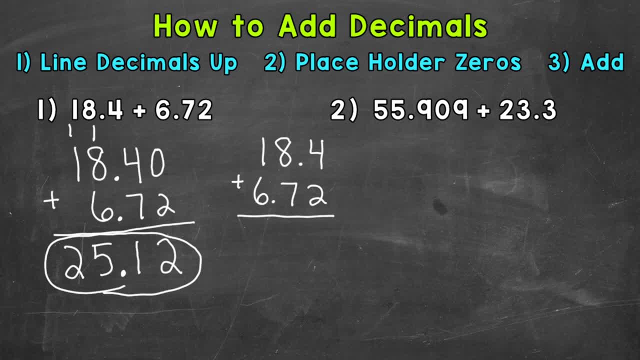 So you can see that the decimals are not lined up. Therefore, our places are not lined up And we're not going to place the decimal correctly in our answer. So this is going to give us something completely different. This is completely incorrect and is a common mistake. 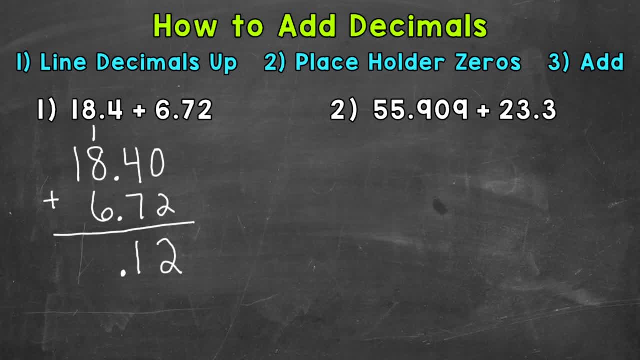 Now we add the ones. 1 plus 8 is 9. Plus 6 is 15. Regroup or carry the 1. Now we add the tenths place. 1 plus 1 is 2. So we get 25 and 12 hundredths. 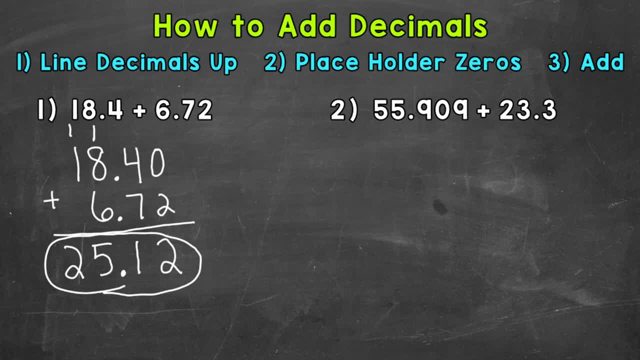 To recap, as far as where we put the decimal in our answer, the decimal should be lined up throughout the entire problem. So we bring it straight down. 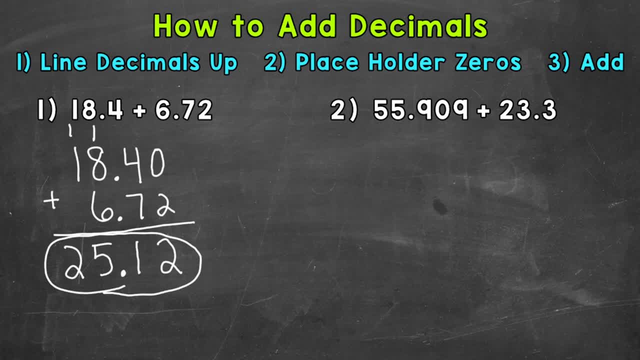 Now before I move on to number 2, I do want to mention a common mistake. And that's going to be lining the digits up. Meaning, for number 1, it would look like this. 18 and 4 tenths plus 6 and 72 hundredths. So 3 digits lined up with 3 digits. So you can see that the decimals are not lined up. Therefore, our places are not lined up. And we're not going to place the decimal correctly in our answer. 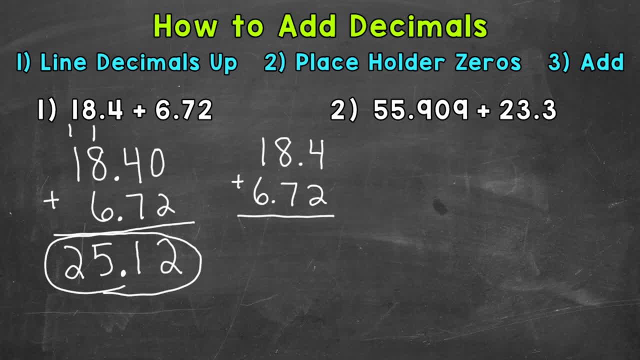 So this is going to give us something completely different. This is completely incorrect and is a common mistake. 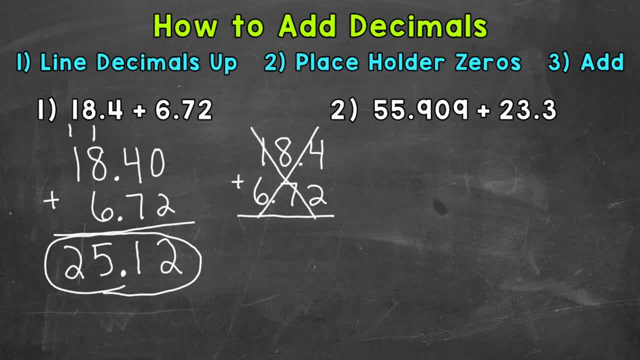 So avoid just lining the digits up. Make sure you have the decimals lined up. Now it is possible that you line the decimals up and then the digits line up as well. Most important part being the decimals are lined up. 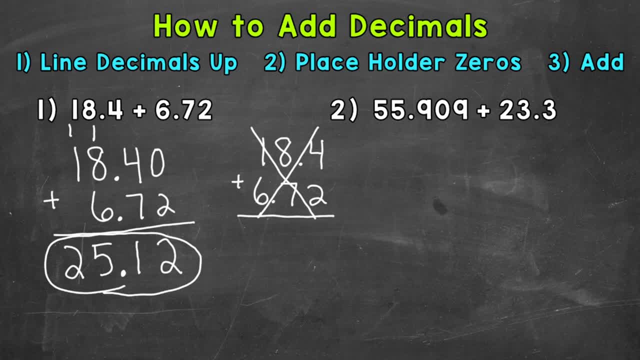 Let's try another example and move on to number 2. Where we have 55 and 909 thousandths plus 23 and 3 tenths. So first step. Line up our decimals. 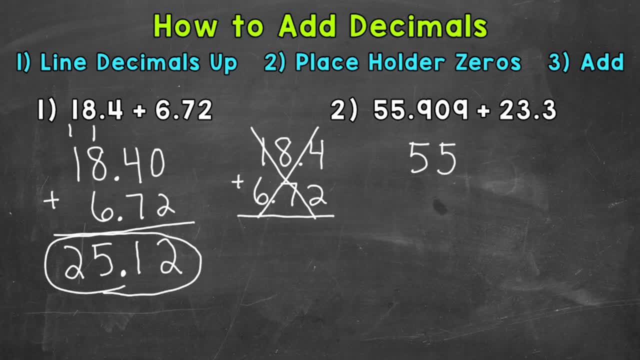 So 55 and 909 thousandths plus 23 and 3 tenths. So we can use placeholder zeros to line this up a little better. So we can place some zeros to the right of 23 and 3 tenths. Remember, zeros to the right of a decimal. Do not change those. Do not change those. Do not change the value. That's an equivalent decimal. So we can do that. Our last step. We add.